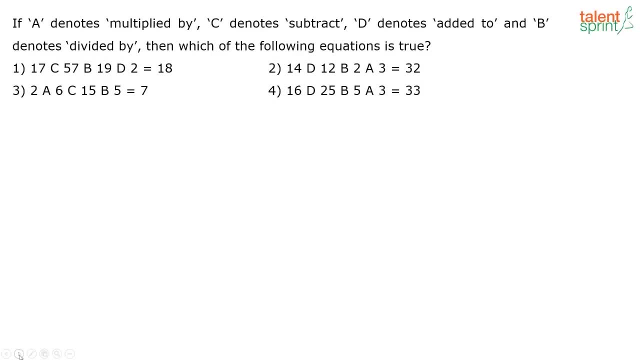 If A denotes multiplied by, C denotes subtract, D denotes added to and B denotes divided by, then which of the following equations is true? Such questions, you just have to go with the trial and error method. Yes, you have to put in check for each option, which is the correct option? which? 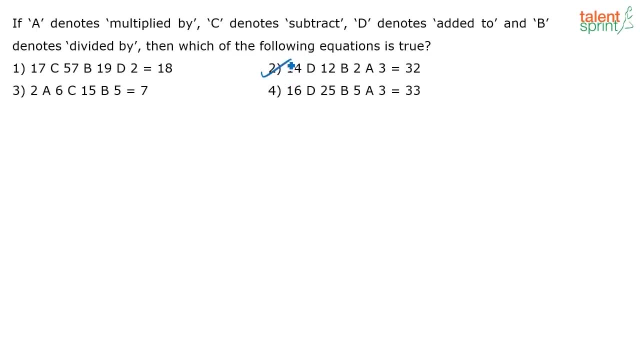 has the right equation. So if you see the correct answer, you will get it as option 2.. So what does option 2 say? 14D12,. what is D? D is nothing but added to add right and B is nothing but divided. 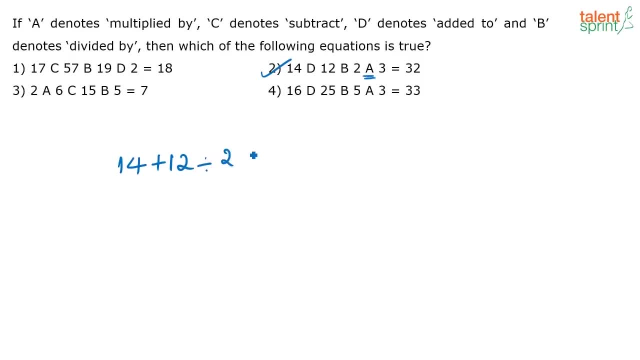 by 2, and A is nothing but multiplied by 3, that is equal to. equal to is what Equal to is the same right. no symbol equal to is the same. So this is what they have given. So you have 14 plus 12. 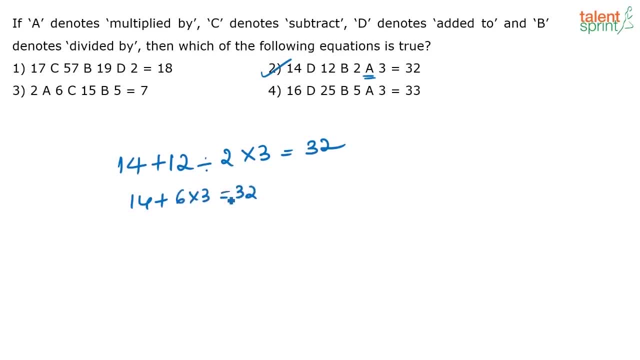 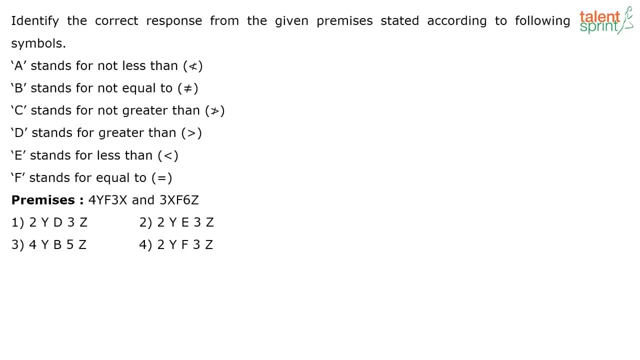 by 2, that is 6,. 6 into 3 is equal to 32.. So here you have 14 plus 18, that is equal to 32, which is the correct one. So the correct answer here is option 2.. Identify the correct response from. 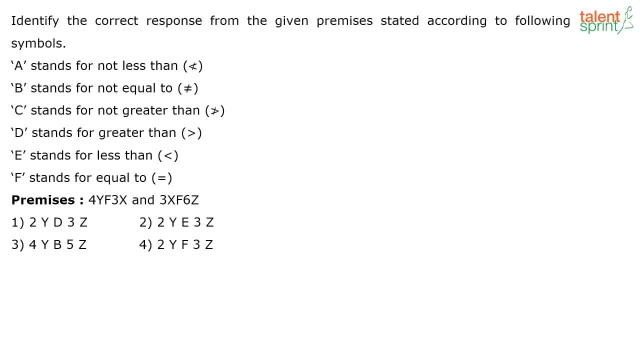 the given premises stated according to the following symbols: Yes, actually the question is very easy. like Vidya says, See what is given here. First thing, that, when you see this question, what will you think? See, they have given what A, B, C, D, E and F stand for, and here they have. 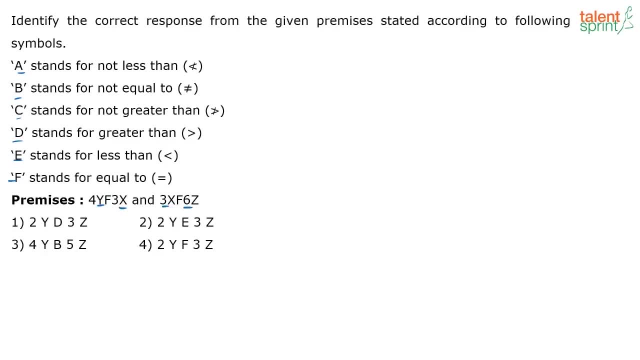 given X and Y, So suddenly you might feel: what are they trying to say? okay, See, X and Y, here are just variables. okay, What do you know? See? you know F stands for So 4YFX, 4YF3X. this means 4Y is equal to 3X. Similarly, when you have 3XF6Z, yes, 3XF6Z. So 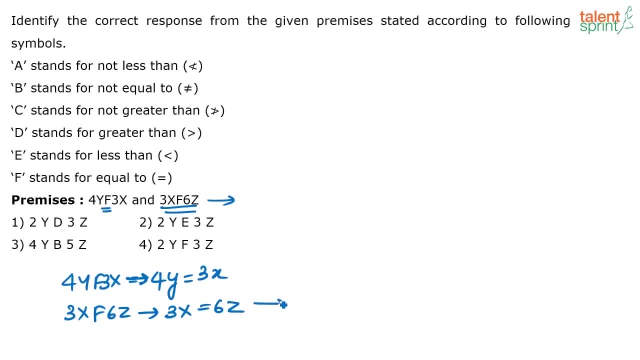 here I can say: 3X is equal to 6Z, or I can say X is equal to 2Z. Here I have: X is equal to 4 by 3Y. So what is the relationship between Between Y and Z? the relationship between Y and Z is 4 by 3Y, that is equal to 2Z, or 4Y, that is. 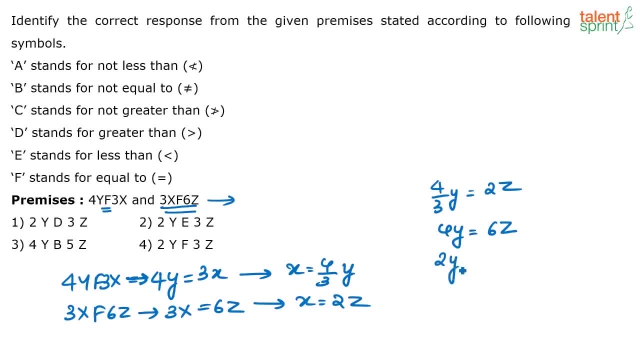 equal to 6Z, right? Or I can say 2Y, that is equal to 3Z. So what is the symbol that is used for equal to 2YF3Z, which is the option 4, okay, Is it clear? A very different question, no, From the. 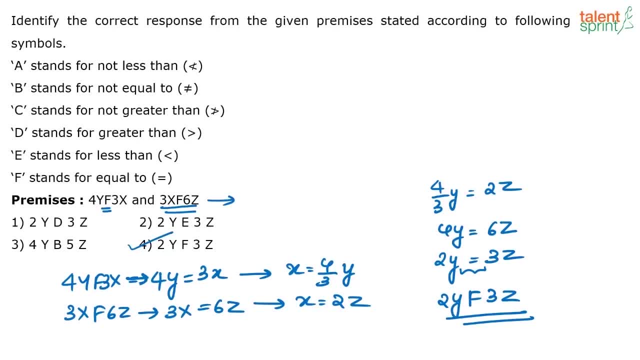 general question types that we have been solving, but very easy. Yeah, it is a very different type of question, but very easy one. So if this question comes, such a question comes in the examination now. I know for sure all of you who have attended this. 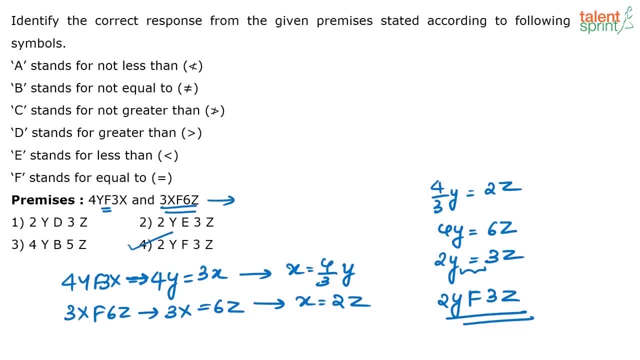 session will get it correct. It was a very easy one. You will not skip it. So correct answer here is 2YF3Z. Yes, you can simply replace 3X with 6Z. Yeah, now the logic is clear too. You can. 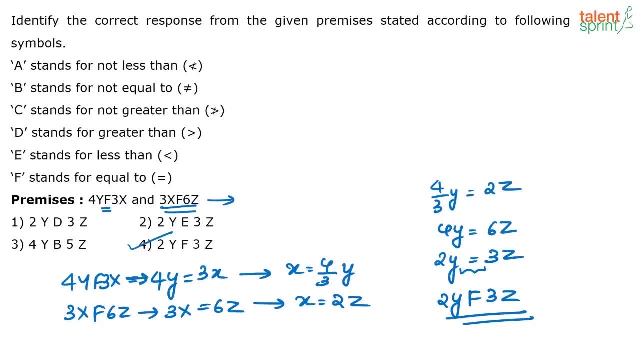 definitely do that. See, you know this F stands for equal to, So instead of that you can replace it here. No issues, I just explained it. That is all okay. Like you say you did not find out, X is: 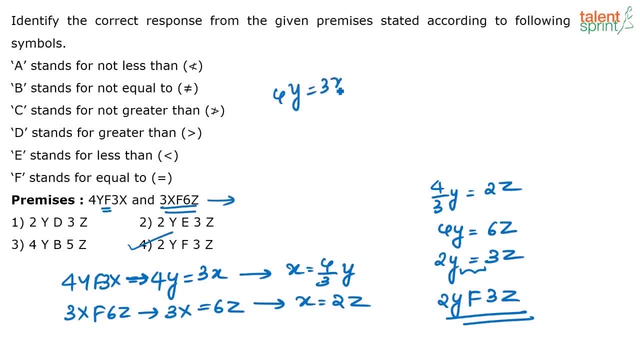 equal to 2YF3Z, So you can simply replace 3X with 6Z. Yeah, now the logic is clear too. You can say: see, you know, 4Y, that is equal to 3X. You know, 3X is equal to 6Z. Directly, you can equate: 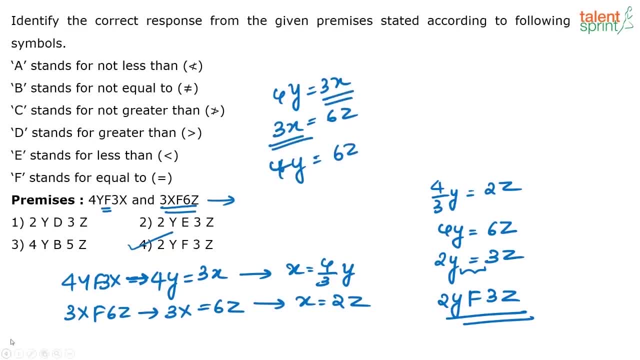 4Y is equal to 6Z, because here 3X and 3X is common. I found out what is the value of X and then equate it. This is actually not required Directly. you can do it with this step, Since it is a new. 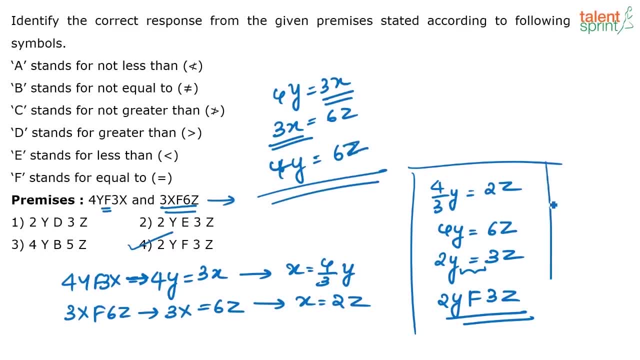 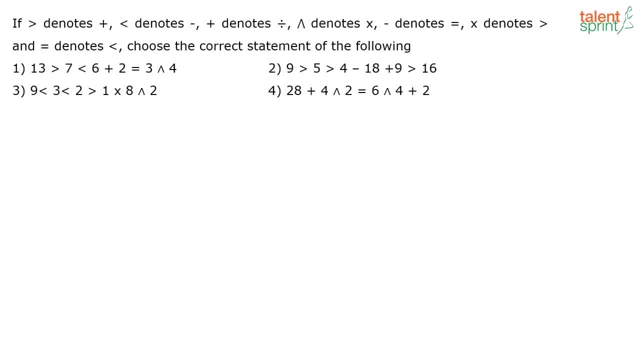 type of question. I just explained it. That is all. You need not go to the fractional part. This part is not even required Directly at this point. you will get the answer 2YF3Z Again. you have to. 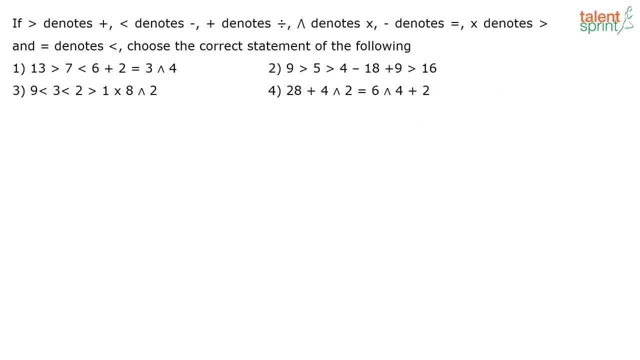 do a trial and error method here to arrive at the answer Here: greater than denotes plus, less than denotes minus, etcetera. Choose the correct statement of the following. So what will the first option be? The first option will be 13 plus 7 minus 6. plus denotes what Divided by 2 equal to. 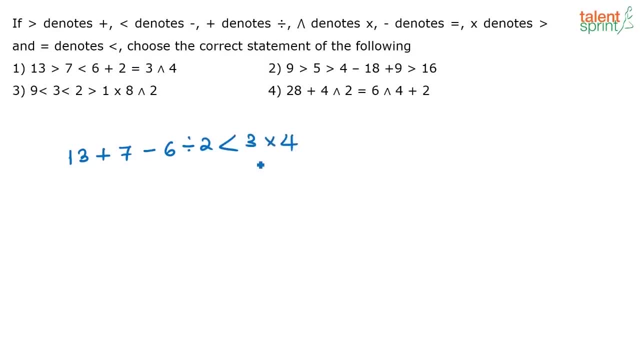 denotes less than 3, 4.. Yes, So you have 13 plus 7, that is 20,, 20 minus 3, that is 17.. Less than 12.. Not possible, right? 17 is not less than 12.. So first option does not follow. 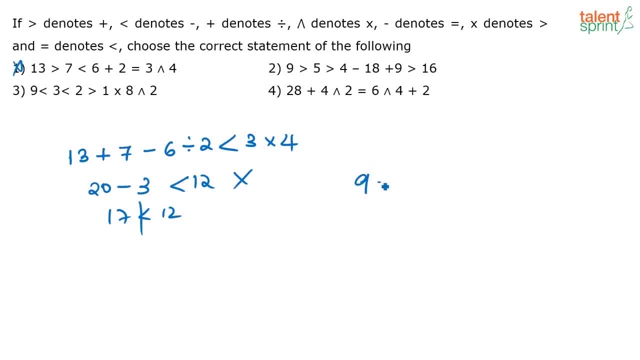 Similarly. now check the second option. What do you have? You have 9 plus greater than is plus 9 plus 5 plus 4 is equal to 18 divided by 9 plus 16.. So this is nothing but 18 is equal to 18.. Option 2 is your correct answer.